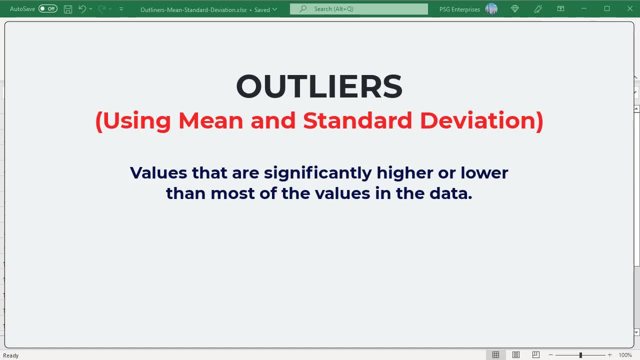 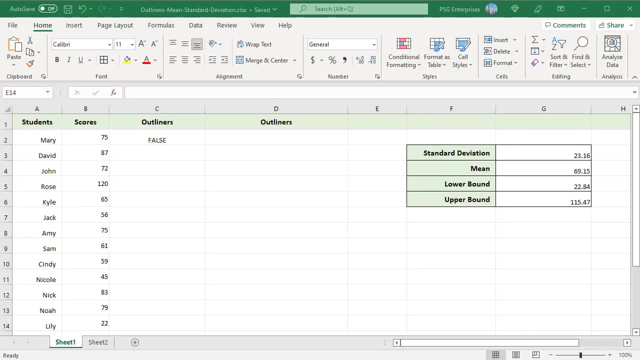 A lower value indicates that the data points tend to be closer to the mean value. A higher value indicates that there is widespread variation in the data points. This can also happen when there are many outliers in the dataset. For example, find the outliers for the scores of students using mean and standard deviation. 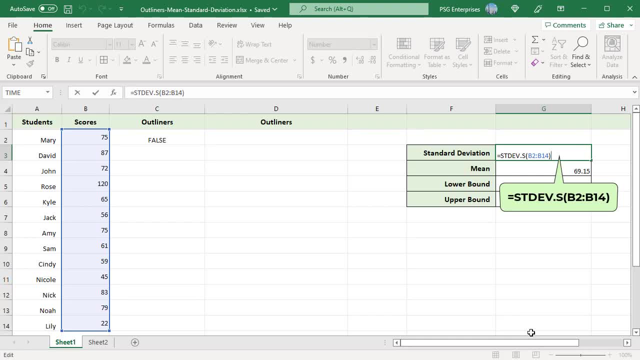 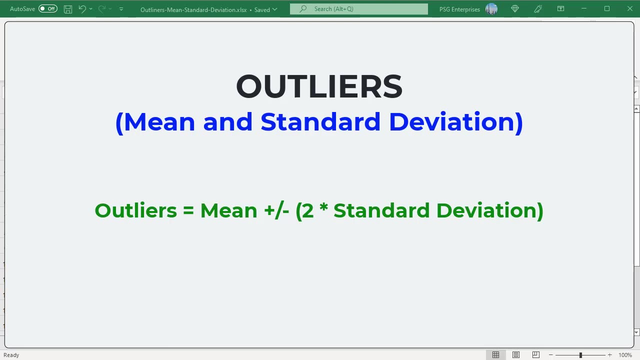 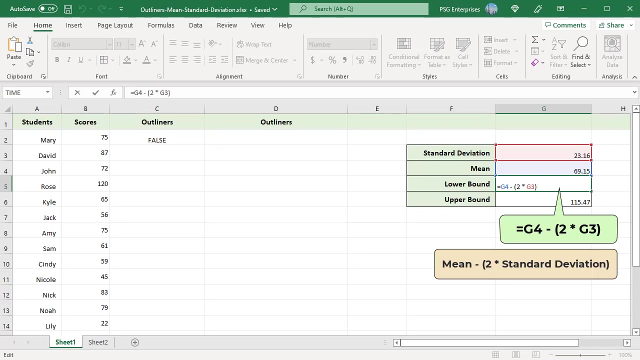 Use the stdevs function to calculate standard deviation. To calculate the mean, use the average function. The values that are two standard deviations away from the mean are the outliers. The lower bound is calculated using this formula: Mean minus 2 multiplied by standard deviation. The upper bound is calculated using this formula: 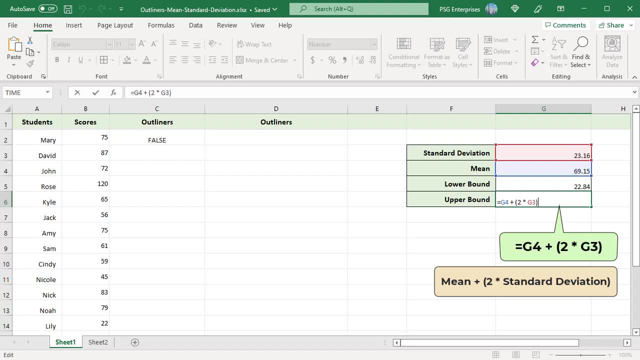 Mean plus 2 multiplied by standard deviation. Outliers are scores that are lower than the lower bound or higher than the upper bound. Use this OR formula to return true for those values that are outliers. This will return true if the score is an outlier and false. 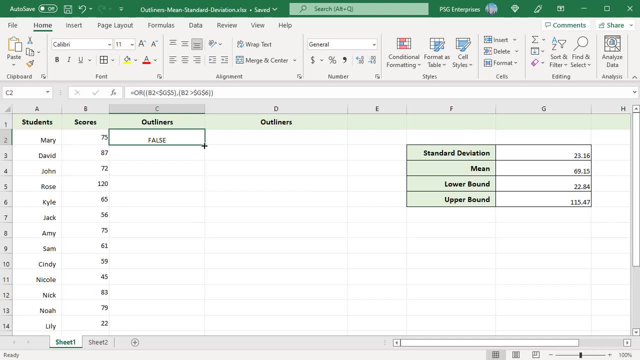 otherwise Copy the formula down: A true indicates an outlier. We have two outlier values: Rose score 120, which is above upper bound, and Lily score 120, which is below upper bound. Rose score 120, which is above upper bound, and Lily score 120, which is above upper bound. and 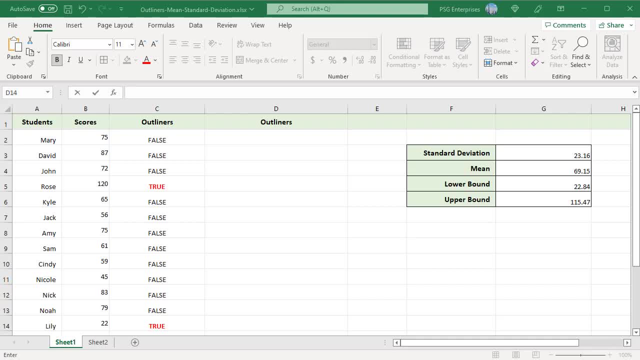 Lily score 120, which is above upper bound, and Lily score 120, which is below upper bound. Instead of just true-false, if you want to mark the outliers as high and low, use a nested IF. Use this formula: The first IF returns low. 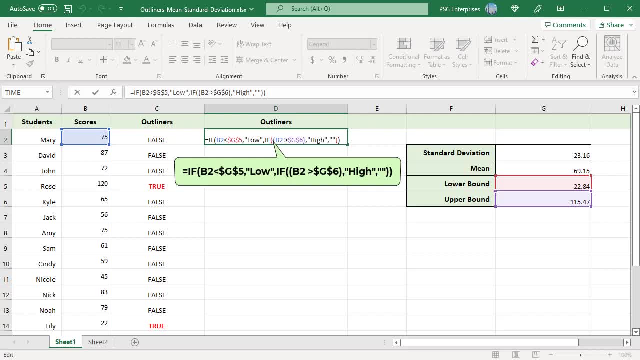 if the score is less than the lower bound, Else the second IF returns high. if the score is greater than upper bound, Else an empty string. Copy the formula down. The outliers greater than upper bound are marked as high and lower bound, Else the second IF returns high if the score is greater. 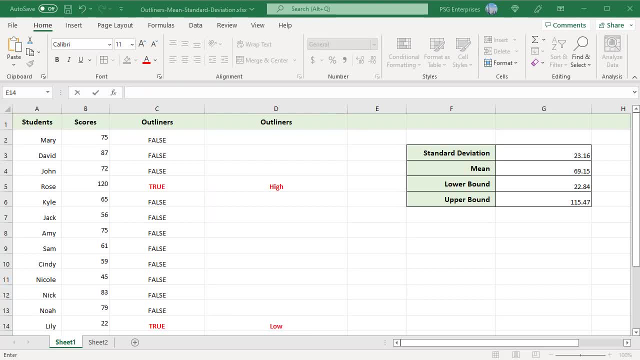 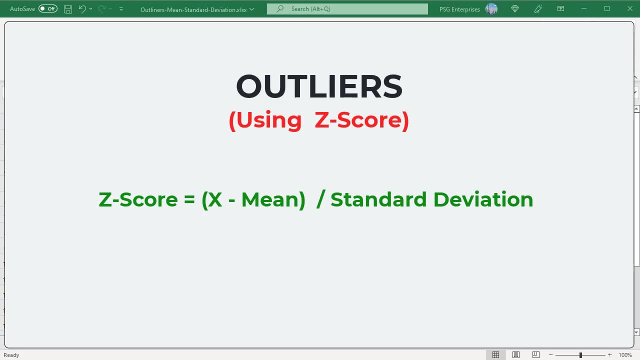 than lower bound, and apart from the lower bound, and less than lower bound are marked as low. Another way of finding outliers is by using the z-score value. The Z-score value, also known as the standard-score, gives an idea of how far a data point is from the mean.